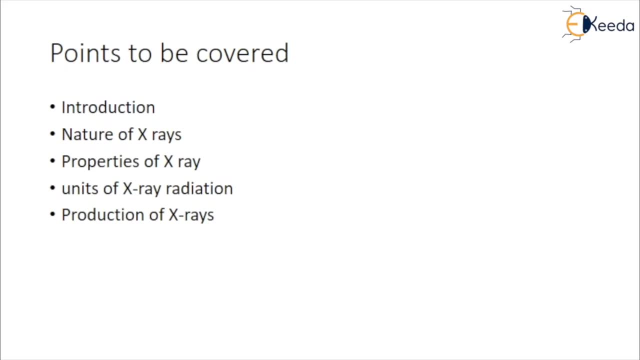 The X-rays in the medical diagnostic region have wavelength of the order of 10 raised to power minus 10 meter. They propagate with the speed of 3 × 10 raised to power, 10 centimeter per second. are unaffected by electric and magnetic fields. 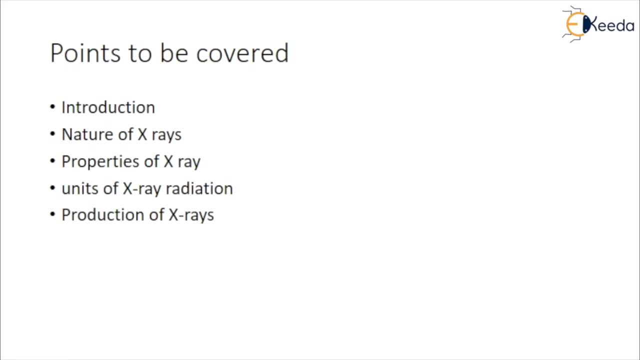 According to the quantum theory, electromagnetic radiation consists of photons, which are conceived as neutrons, which are conceived as neutrons, which are conceived as neutrons, as a package of energy. Their interaction with the matter involves an energy exchange and relation between a wavelength and the photon is given by. E, is equal to h, nu, and it is also. 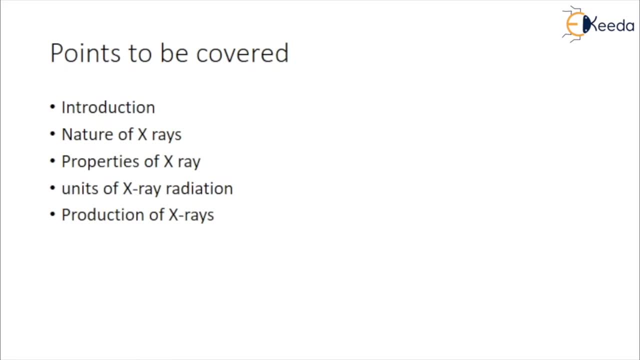 equal to h into c upon lambda, where h is the Planck's constant, c is the velocity of propagation of photons, mu is the frequency of radiation and lambda is the wavelength Properties of x-ray. Because of the short wavelength, the extreme high-energy x-rays are able to penetrate through. 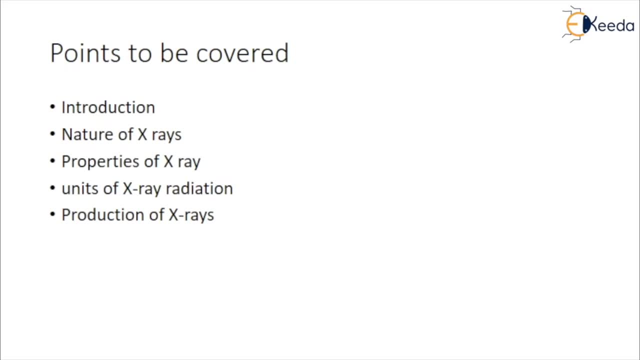 the body. X-rays also produce fluorescence in certain materials to help them emit light. Fluoroscopic x-screens and intensify screens have been constructed on the basis of these properties. X-rays affect photographic film in the same way as ordinary visible light. 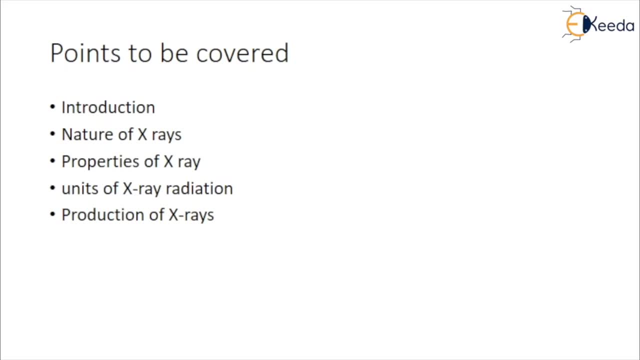 Units of X-radiation. The International Commission on Radiological Units and Measurements has adopted a new approach to x-ray radiation. It adopted RONC-10 as a measure of quantity of x-radiation. This unit is based on the ability of radiation to produce ionization is abbreviated as capital R. One R is the. 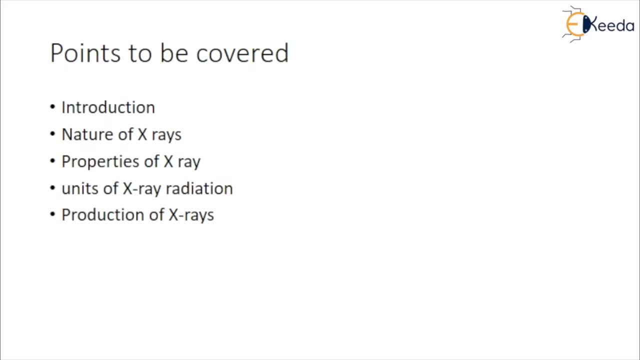 amount of x-radiation which will produce 2.08 into 10, raised to the power, 9 ions pairs per cubic centimeter of air at standard temperature, 0 degrees Celsius and at pressure, 760 mm Hg at sea level. Other units derived from RONC-10 are: milli-RONC-10 is equal to 1 upon 1000 R and micro-RONC-10. 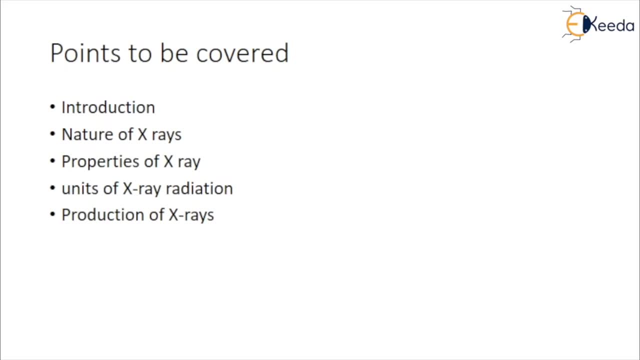 is equal to 10, raised to the power minus 6 R. The unit of x-radiation has been based on the ionization produced by the x-rays and not on the other effects like blackening of the photographic film, due to the ease and accuracy with which the ionization in the air can be measured. 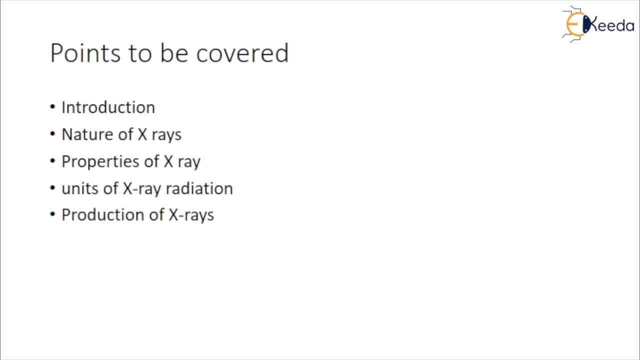 Production of X-rays. X-rays are produced by the X-ray machine. X-rays are produced by the X-ray machine. X-rays are produced whenever electrons collide at very high speed with the matter and thus suddenly stop. The energy possessed by electrons appears from the site of the collision a. 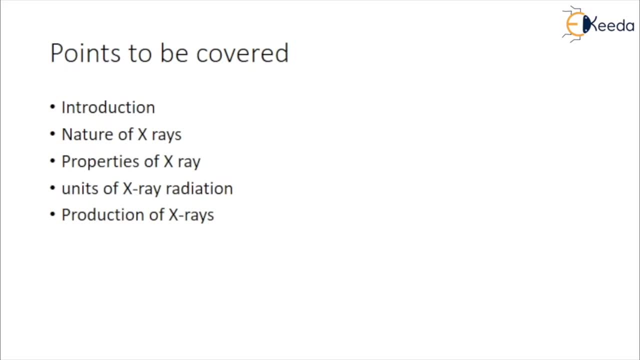 parcel of energy in the form of highly penetrating electromagnetic waves of many different wavelengths, which together form a continuous spectrum. X-rays are produced in a specially constructed glass tube which basically comprises a source for the production of electrons. An energy source is produced by the X-ray machine. X-rays are produced by the X-ray machine. 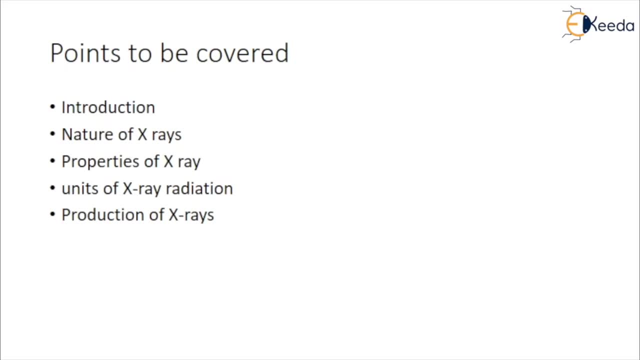 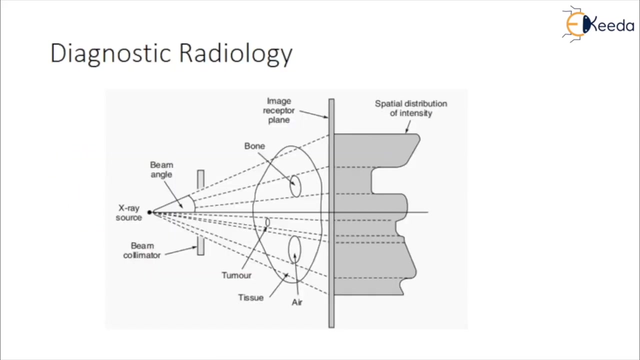 X-rays are produced by the X-ray machine. X-rays are produced by the X-ray machine. worry, And the solution is the efficiency of three. step this Here it makes sense, became It isreh The value DLC, He It did another. Different types of lung infections are accompanied by characteristic changes which often enable 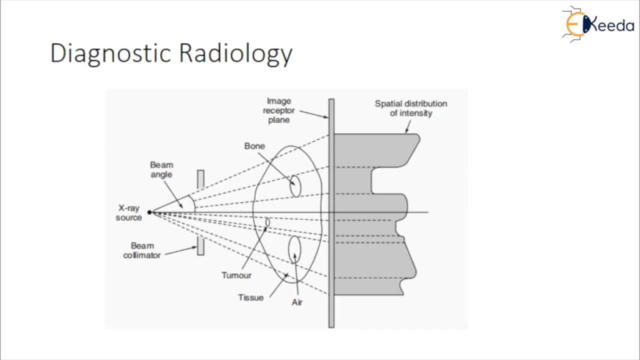 a diagnosis to be made from the location, size and extent of the shadow. All the larger organs of the body can be examined by visualizing the associated vessels, and this technique is called angiography. The examination is designed according to the organ examinants, for example, coronary angiography. 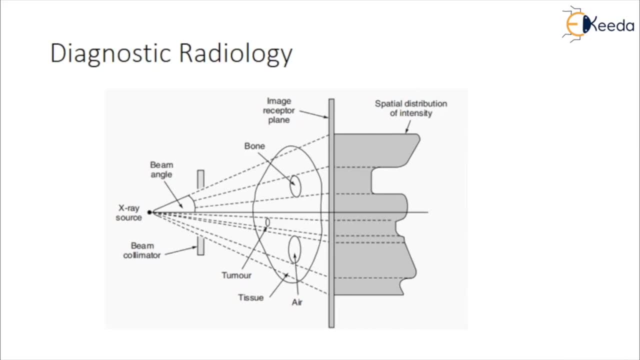 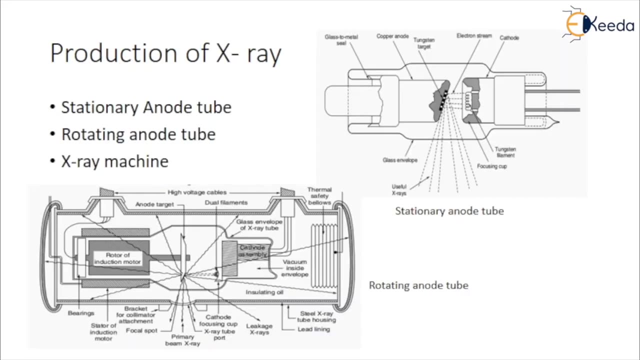 – the coronary vessels of the heart angiocardiography – the heart, the cerebral angiography and the brain. Production of X-ray Stationary Anode Tube. The normal tube is a vacuum diode in which the electrons are generated by thermionic emission from the filament of the tube. 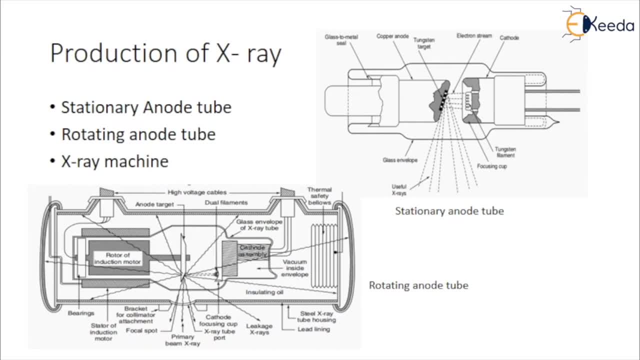 The electron stream is electrostatically focused on the target, on the anode, by means of a suitably shaped cathode cup. The kinetic energy of the electrons impinging on the target is converted into anode X-rays. Most electrons emitted by the hot filament become current carriers across the film. 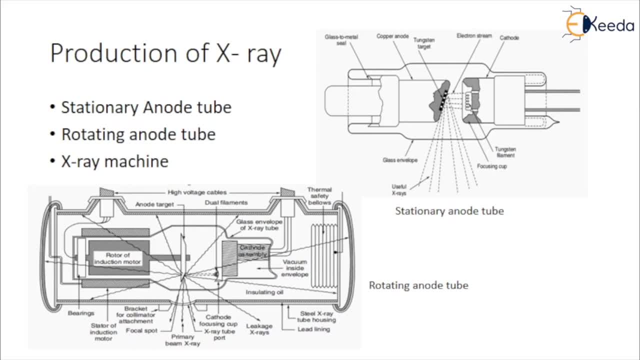 It is therefore possible to independently set the tube current by adjusting the filament temperature. Some X-ray tubes function as a triode, with a bias voltage applied between the filament and the cathode cup. The bias voltage can be used to control the size and shape of the focal spot by focusing. 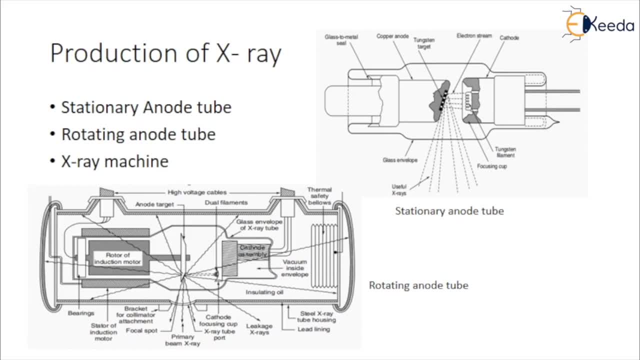 on the electron beam in the tube. The filament is a closely wound helix tube. The helix of a tungsten wire is about 0.2 mm thick, the helix diameter being about 1.0 to 1.5 mm. 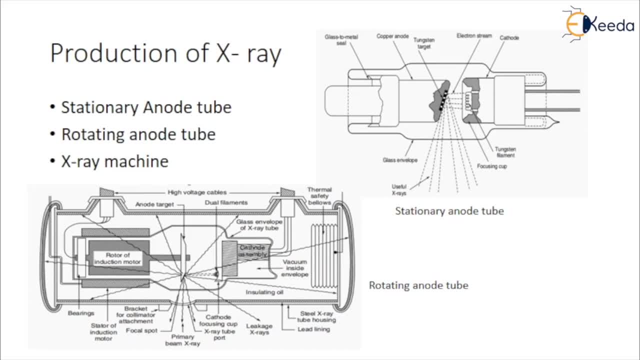 The target is normally compromised- of a small tablet of tungsten about 15 mm wide, 20 mm long and 3 mm thick, soldered into a block of copper. Tungsten is chosen since it combines a high atomic number, 74, making it comparatively 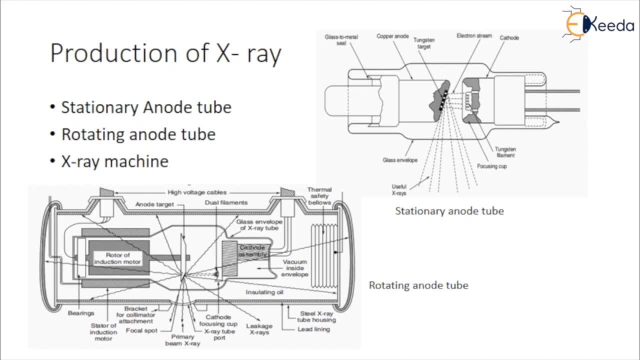 efficient in the production of X-rays. Copper, being an excellent thermal conductor, forms the vital role of paring the heat rapidly away from the tungsten target. The heat flows through the anode to the outside of the tube, where it is normally removed. 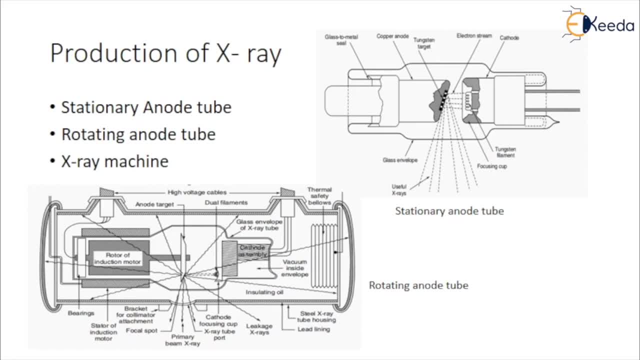 by convection. Generally, an oil environment is provided for the convection. current cooling rotating anode tube. With an increasing in the need of radiology for more penetrating X-rays, requiring higher the tube voltages and current, the X-ray tube itself becomes a limiting factor. 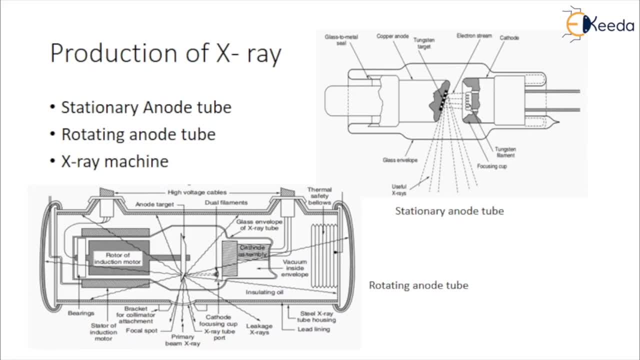 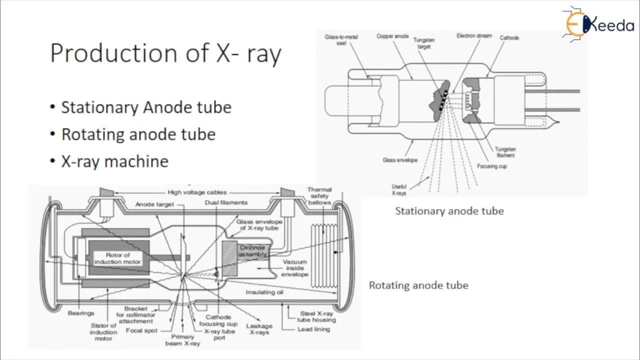 This is primarily due to heat generated in the anode. The heat capacity of the anode is a function of focal spot area. The adsorb power can be increased if the effective area of the focal spot can be increased. This is accompanied by the rotating anode type of X-ray tubes. 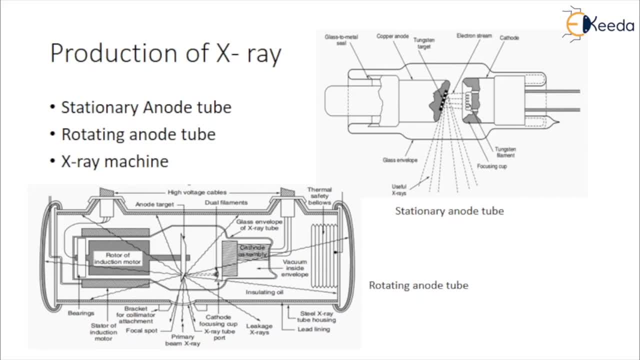 The tubes with rotating anode are based on the removal of the target from the electron beam before it reaches to higher a temperature under the electron beam. under the electron beam bombardment, and rapid replacement of it by another, cooler target. The construction of typical rotating anode X-ray tube. 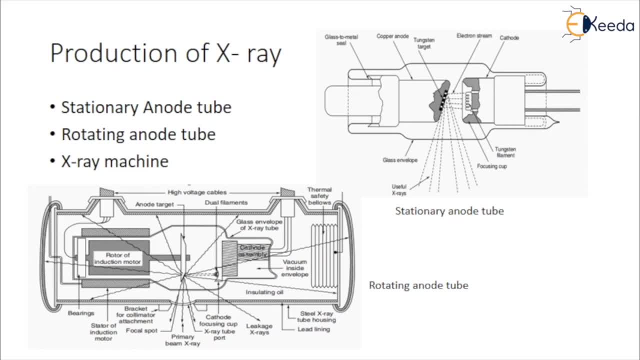 The anode is a disk of tungsten or an alloy of tungsten and 10% rhenium. The alloy helps to reduce the changes in the anode track due to stress produced in the track as a result of rapidly changing temperature. The anode rotates at a speed of 3000 to 3600 or 9000 to 10,000 rpm. 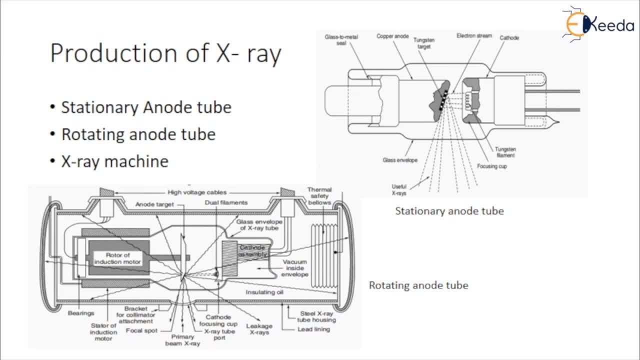 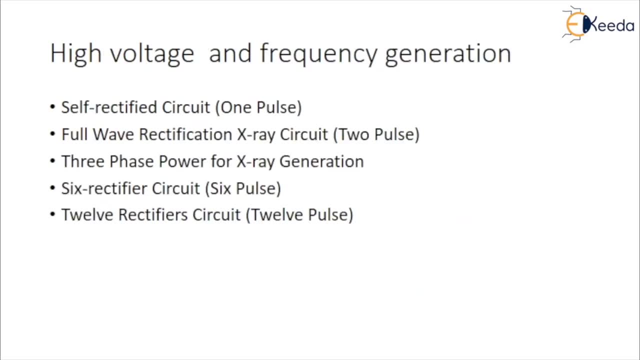 The tungsten disk that represent the anode has a bevelled edge that may vary from 5 degree to 20 degree. High voltage generation and frequency generation Voltages in the range of 30 to 200 kilowatt can be required for the production of X-rays for diagnostic purpose. 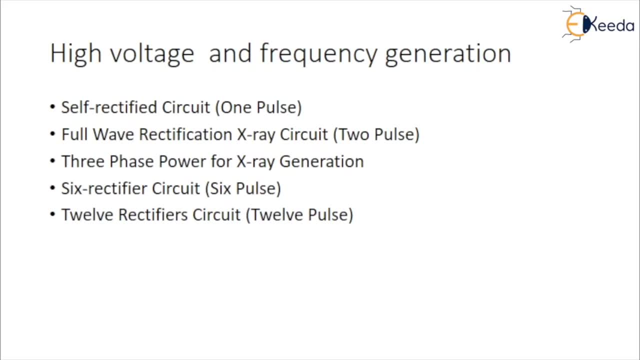 They are generated by an high voltage. A high voltage transformer is used so that voltage applied to primary winding are small in comparison to those taken from the secondary winding. The ratio will be in the range of 1 is to 500, so that the input 250 volt will produce an output of 125 kilovolt. 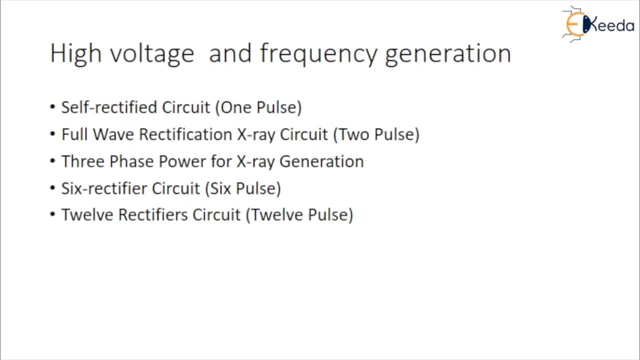 The high tension transformer assembly is immersed in a special coil which provides high level of insulation. Self rectifier circuit, One bulb. A high voltage is produced by using step-up transformer whose primary is connected to an auto transformer. The secondary of HD transformer can be directly connected to the anode of the X-ray tube, which will conduct only during the half cycles when the cathode is negative with respect to the anode. 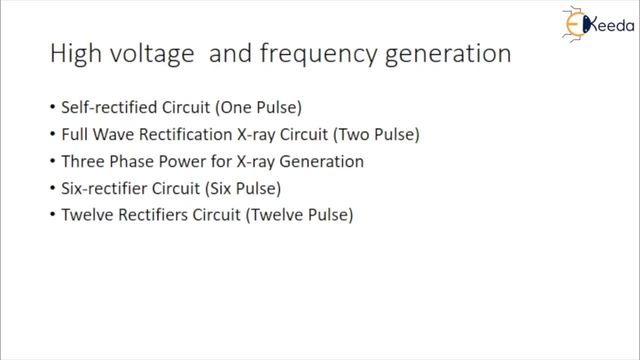 These machines have maximum current of about 20 milliampere and voltage of 100 kilovolt. Full wave rectification: Two pulse In a self rectified unit. X-rays are produced in a burst and considerable amount of exposure time is lost during the half cycle when the X-ray tube is not conducting. 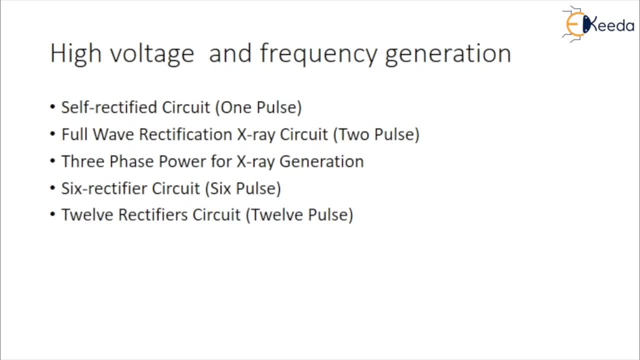 Full wave bridge rectifier circuit, The exposure time for the same radiation output is reduced by half in comparison to the one pulse system. This circuit produces X-rays during each half cycle on the applied sinusoidal 50 hertz main supply voltage, as the anode will be positive with respect to the cathode. 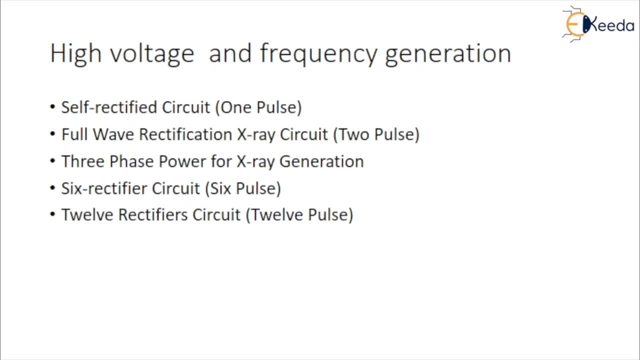 Over both the half cycles. Three phase power for X-ray generation. X-ray in circuits based on the single phase supply provide a pulsating voltage to the anode. These type of voltage waveforms, when used to accelerate electrons in the X-ray tube, results results in the disadvantage 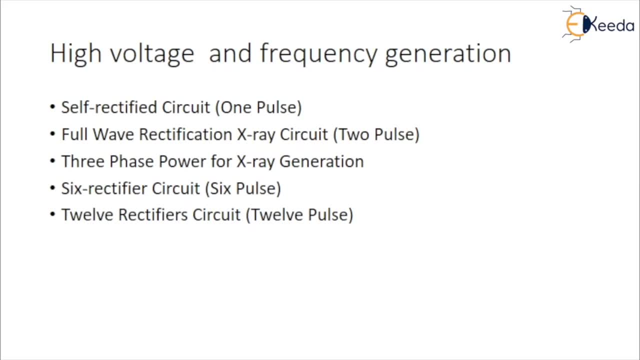 The intensity of radiation produced is lower because no radiation is generated during a large portion of the exposure time. Six rectifier circuit, Six pulse, Simple Six rectifier pulse circuit using three phase power supply. The primary supply is delta connected, whereas the secondary is star connected. 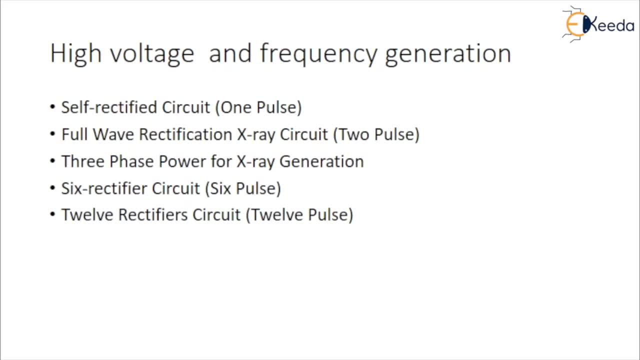 The secondary is connected to a six rectifier arrangement for full wave rectification and the three phase transformer output voltage Twelve rectifier circuit. Now the further refinement of the three phase generation is to use a combination of both star and delta winding on the secondary side. 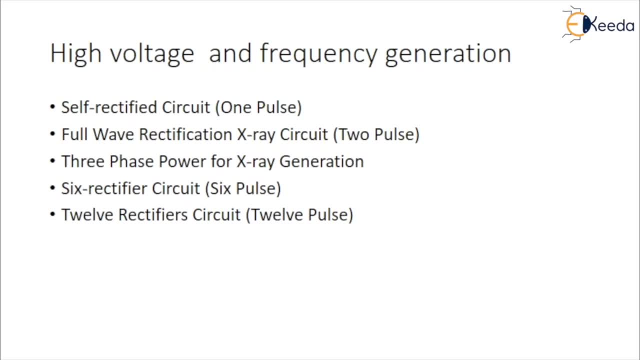 High frequency generator. Modern X-ray machines Make use of high frequency generators for producing high voltage. The high frequency used in these generators varies from 500 hertz to 20 kilohertz- High frequency generated by you by first converting the 50 hertz power lines frequency into a high frequency oscillations in the converter circuit. 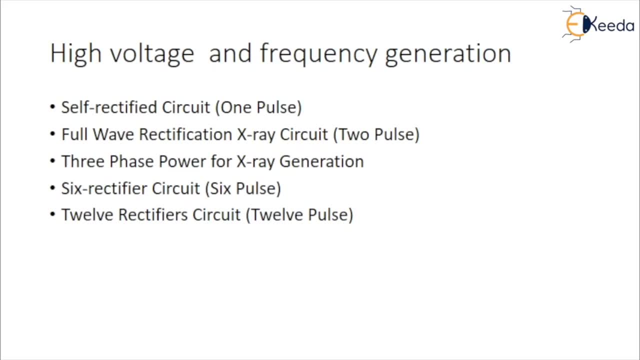 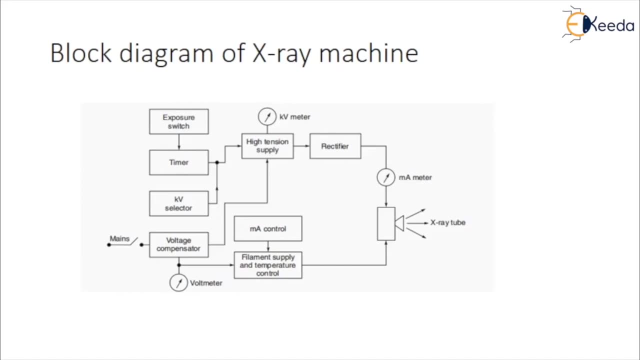 The frequency conversion permits the use of much smaller transformers than those required with conventional equipment. The block diagram shows the basic X-ray machine subsystem. There are two main parts of the circuit. One of them is producing high voltage which is applied to the tubes, anode and the cathode, and high voltage tape up transformer followed by a rectification. 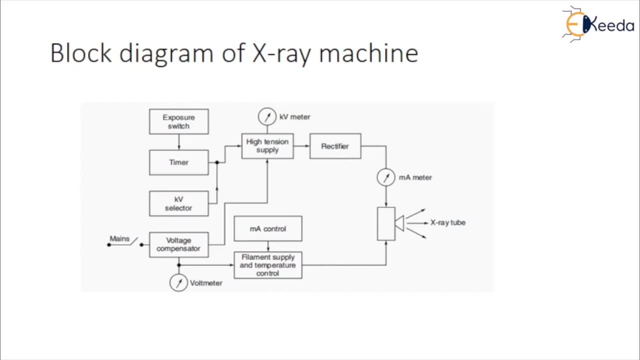 The current through the tube follows the HD pathway and is measured by a milliampere meter. The kilo volt sector selector switch facilitate change in the voltage between exposures. The voltage is measured with the help of kilo volt meter. The exposure switch controls the timer and does 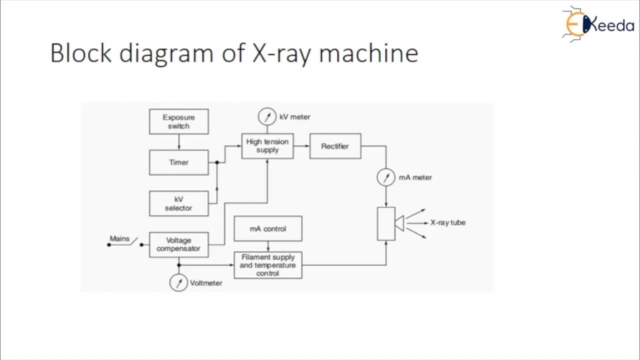 The duration of application of kilo volt. The compensator of my main supply voltage, 230 volt variation voltage compensator, is included in the circuit. The second part of the circuit concern the control of heating X-ray tube filament. The filament is heated with 6 to 12 volt of AC supply at a current of 3 to 5 ampere. 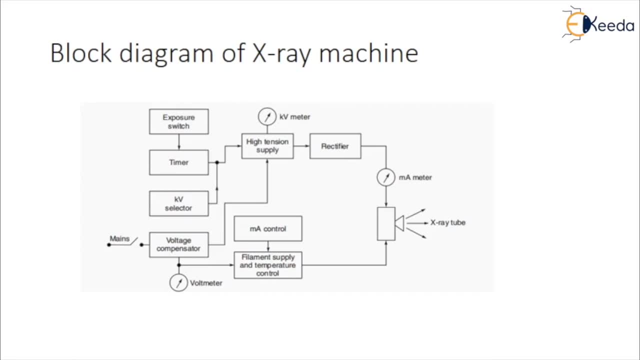 The filament temperature determines the cut tube current of or milliampere. Therefore The filament temperature control has an attached milliampere selector. The filament current is controlled by using, in the primary side of the filament transformer, Variable choke or a rheostat is used. 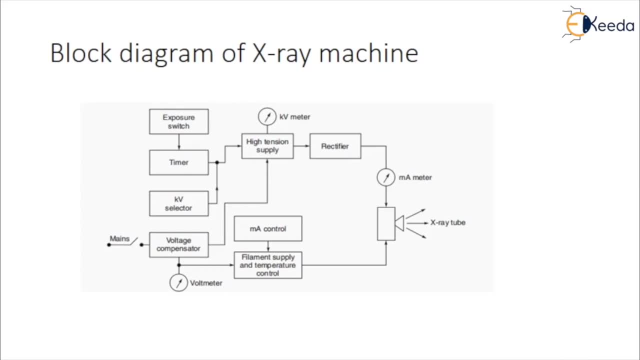 The rheostat provides a stepwise control of milliampere and is most commonly used in modern machines. The preferred method of providing high voltage DC to the anode of the X-ray tube is by use bridge rectifier using four valve tubes or solid state rectifiers.